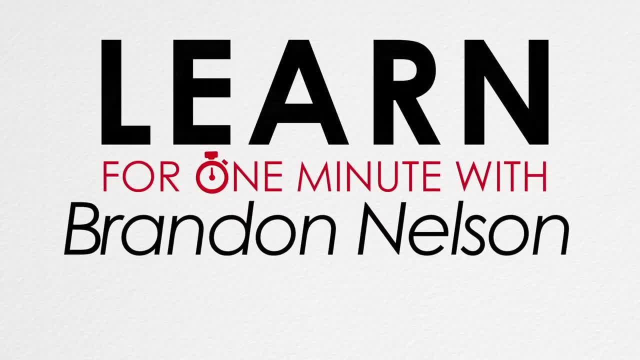 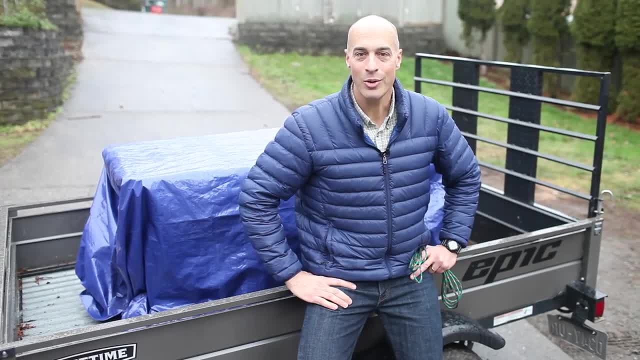 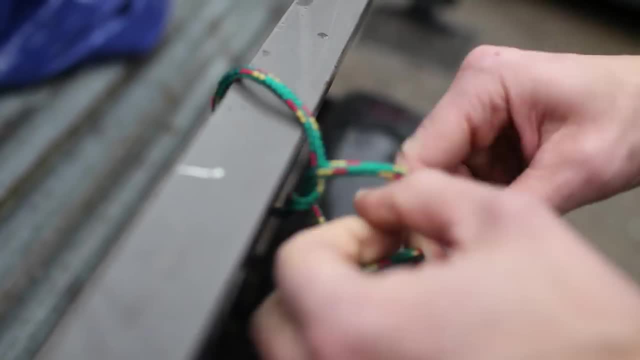 Hey everyone, Brandon Nelson, and in one minute I'm going to show you the two knots you need to know to tie down any load. Here's how most people tie the first knot: They put the rope through and then they just start making tangles until it looks like something that won't come undone, and they hope for the best. 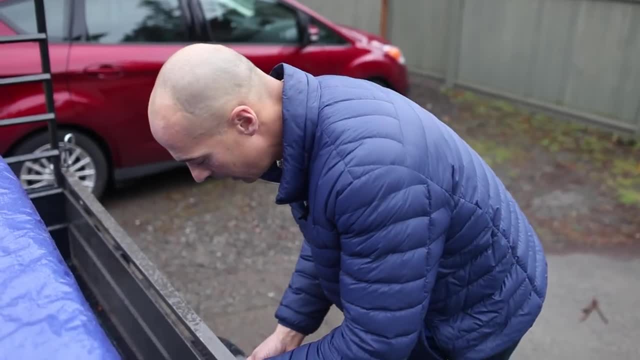 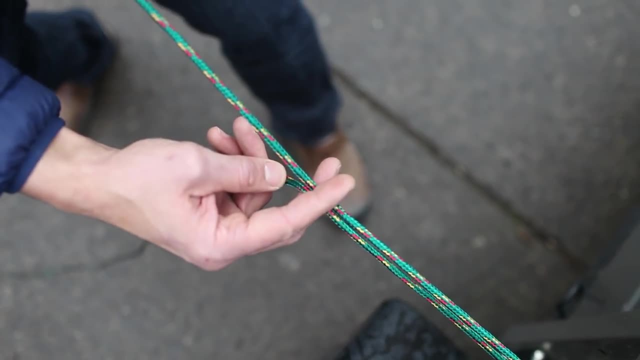 Now here's how you should be doing it. This knot is called a GE. Now watch what I do here. I'm going to come from underneath, bring some of the rope back, then pinch it with my fingers. fold this end over. 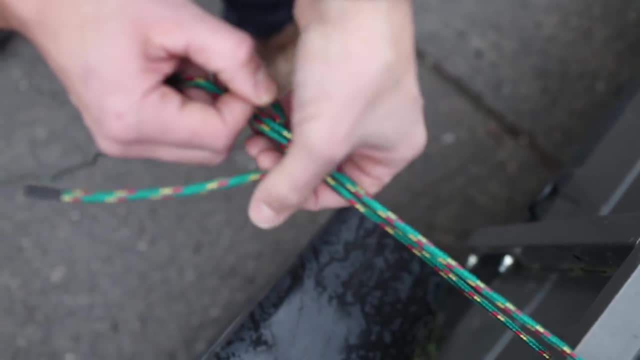 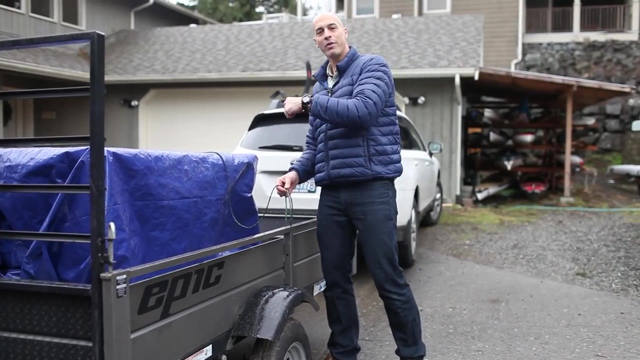 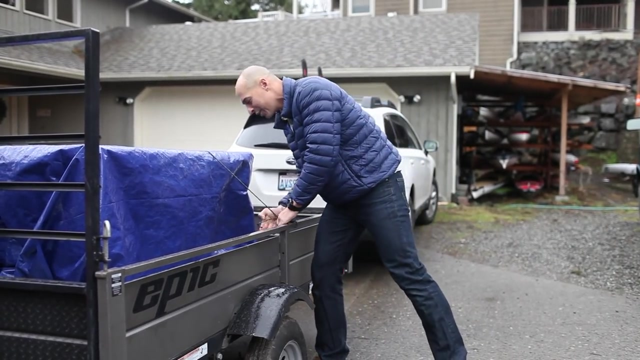 Now I'm going to wrap it twice around those two lines and put a loop through, and that's it. Then I'm going to pull it tight against the trailer. We've got our hitch over there, so we come across the top of the load and then again, what most people do is pull as tight as they can and then make some new tangles and hope for the best. 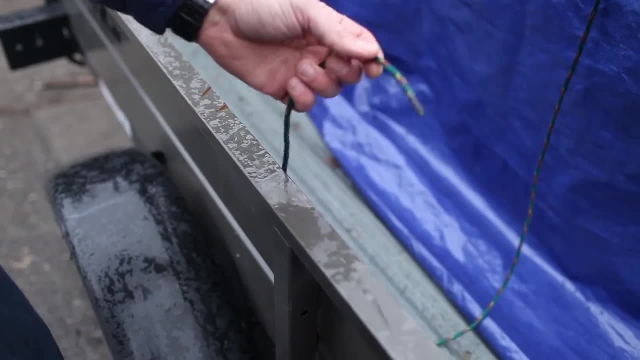 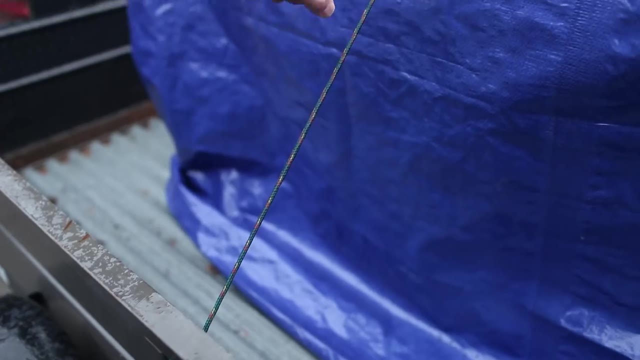 All right, but here's what we're going to do. We're going to tie what's called a trucker's hitch. All right, take the end of the rope and pass it underneath again, and then we're going to come back up to real close to the load. grab some of this rope, make three twists, okay. 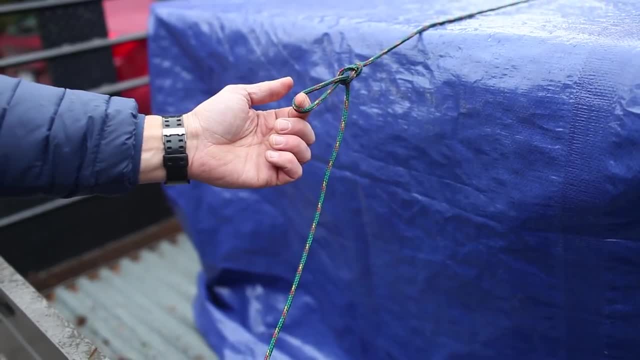 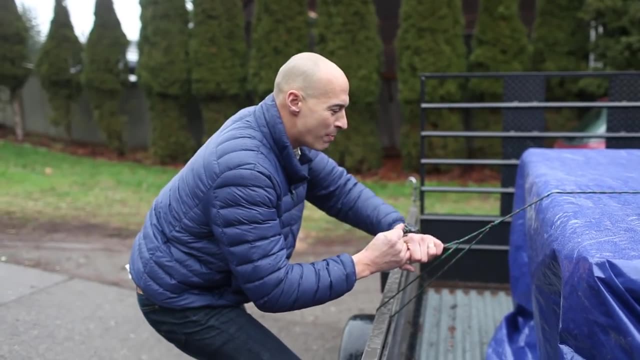 Then we're going to pull a loop through. That loop is now like a pulley for us. Now we take the end of our rope and come through that loop, We've got a three-to-one mechanical advantage where we can really pull it tight. 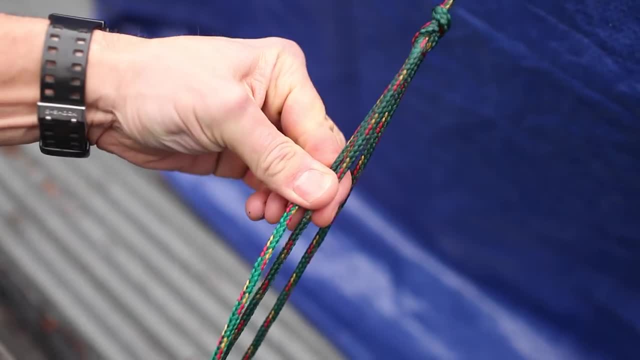 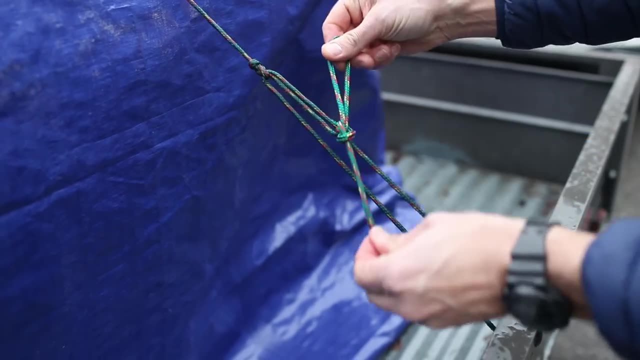 We've got it super tight. I'm just going to pinch right here And make a half hitch And the last step is to take that end and put another half hitch on it to lock it. Now here's the best part: When you're all done, watch how smoothly these knots come apart. 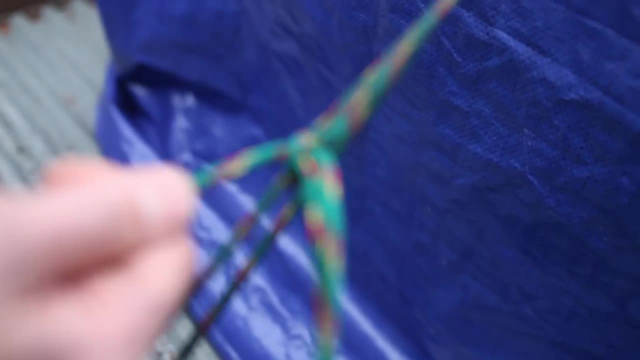 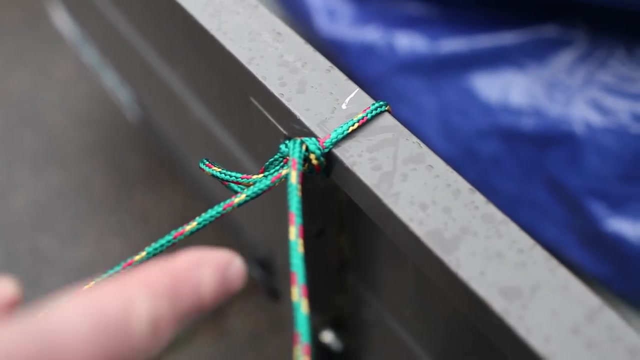 For the trucker's hitch. we take that lock off, then we pull the first loop, pull our rope through, pull the second loop. Now back to our first knot. same thing. You just take that tail, pull it, knot comes right out. 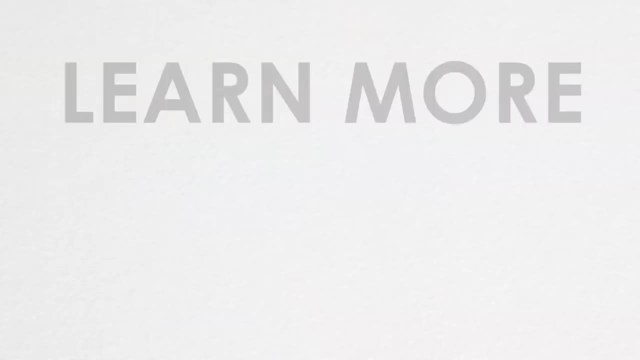 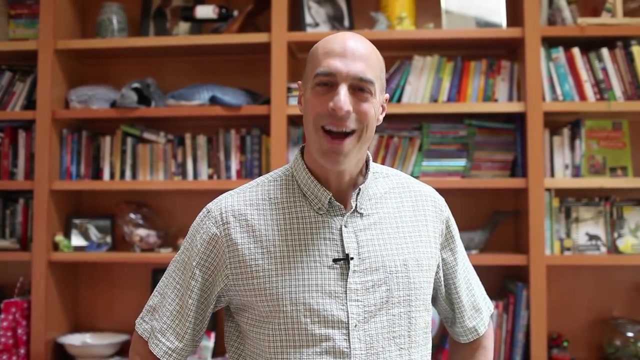 This has been Brandon Nelson for one minute. I'll see you next time. What do you want to learn in one minute? Comment below or email me at brandon at brandonnelsoncom.